and world workshops are introduced to name mammals and we get to select a few of them to focus on. here. However, many of us will be David Mitchell. I'm kicked out of school or the THATdate for today and will give a brief presentation. For more info, check out our search. 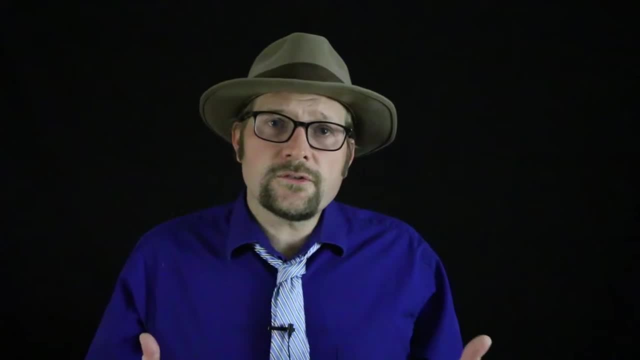 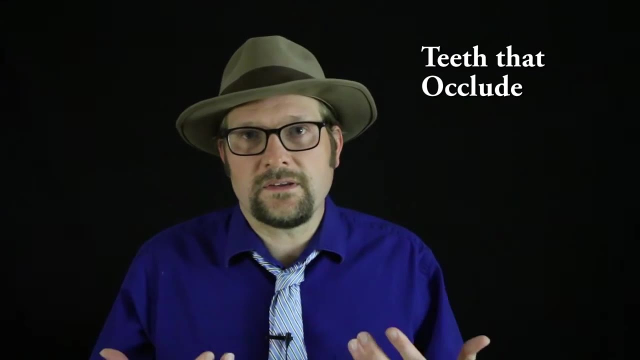 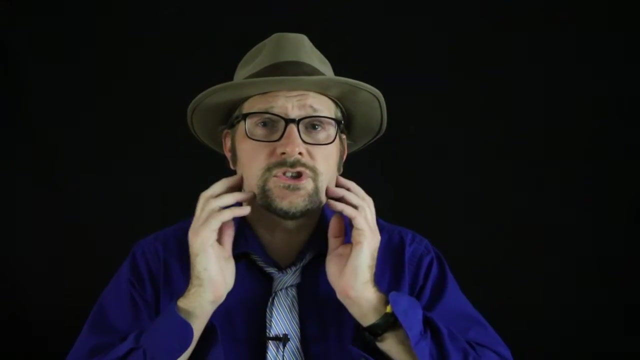 hopefully can be preserved as fossils. The first trait that is shared by all mammals are teeth that occlude and feature a series of characteristic teeth: incisors in front, canines for piercing, premolars and molars for chewing in the back. 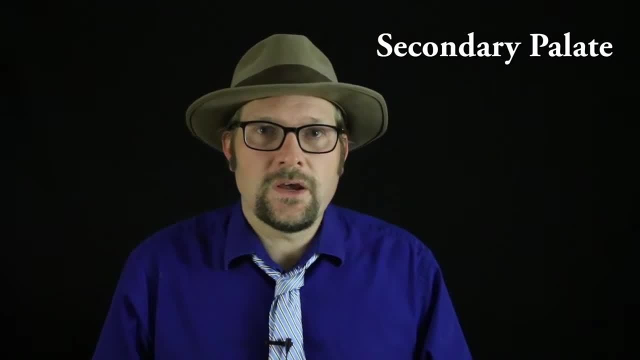 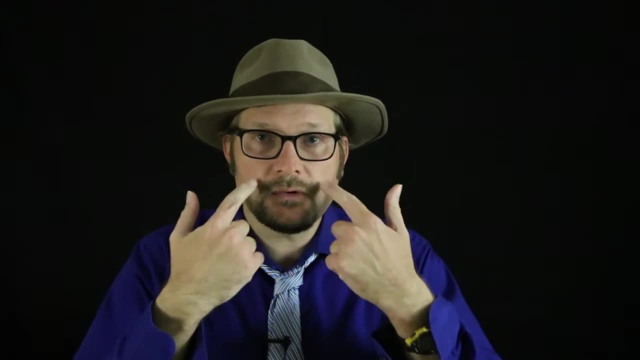 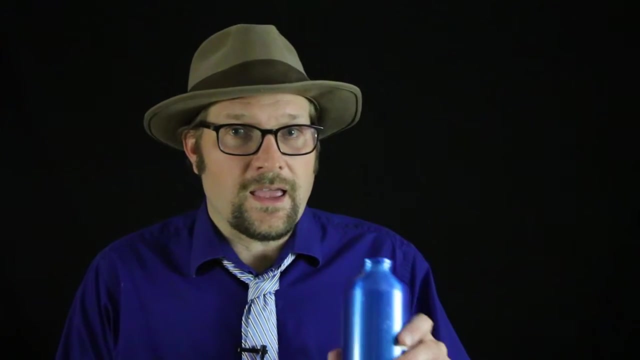 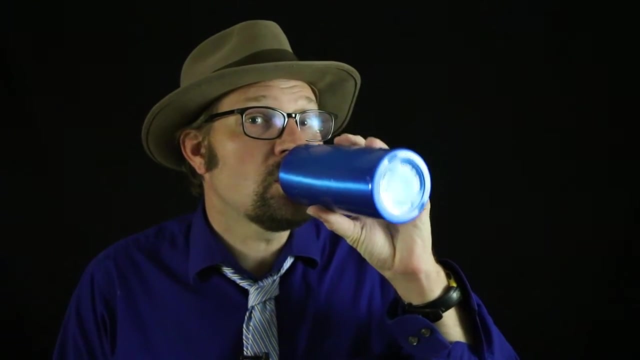 The second trait is a secondary palate which caps the roof of the mouth and separates the passageway for respiration through the nose and eating through the mouth. The secondary palate allows mammals to both drink and eat at the same time as they breathe. 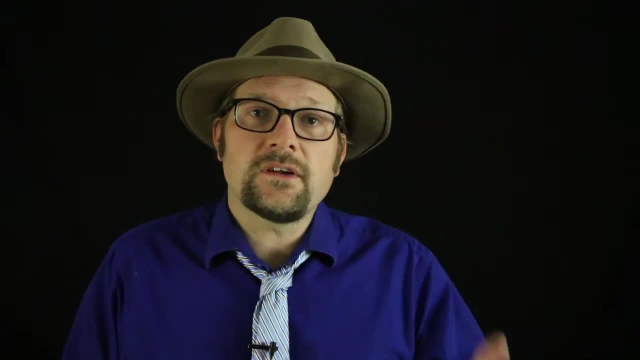 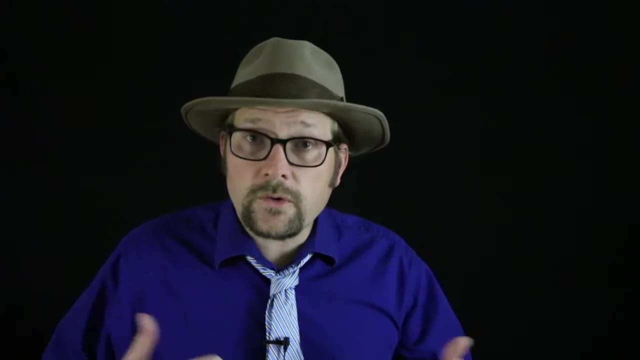 In suckling infants. this is really important, as it allows mammals to suck at the nipple or gland while also being able to breathe. Several other traits are also shared by all mammals. They are also characteristic of mammals: their erect gait, their larger brains and. 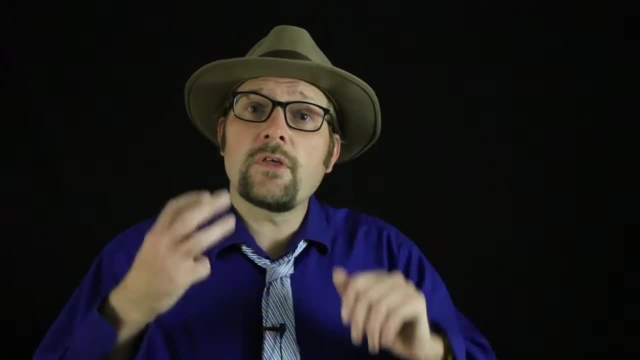 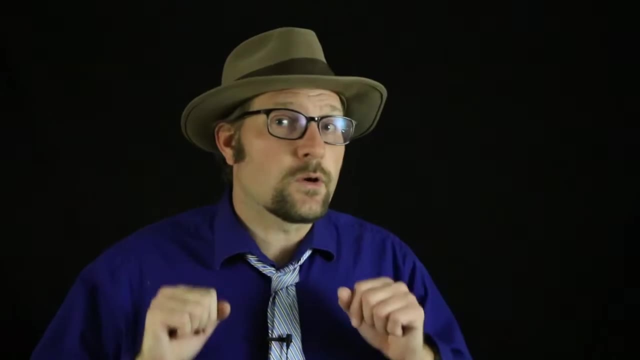 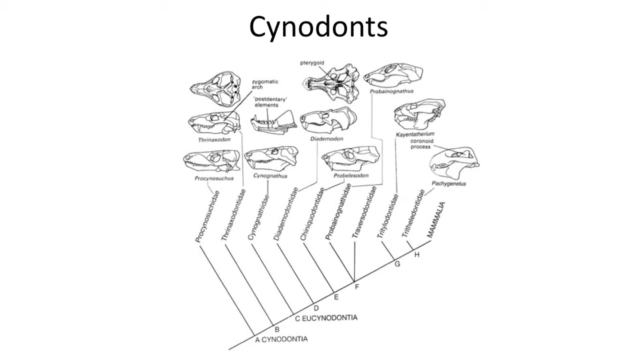 one trait that we will look at in detail is a development of three middle ear bones from a series of jaw bones near the joint between the skull and lower jaw. Cynodonts as a group are a very diverse group of synapsid reptile-like mammals that survive. 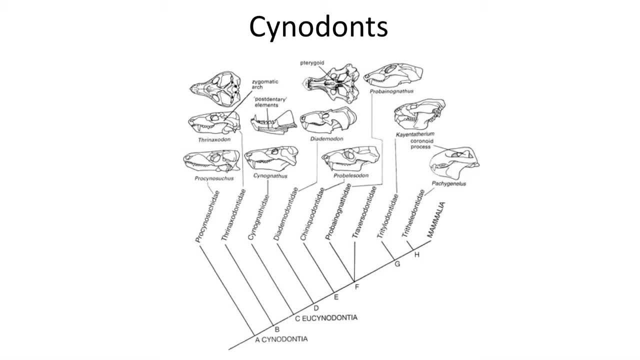 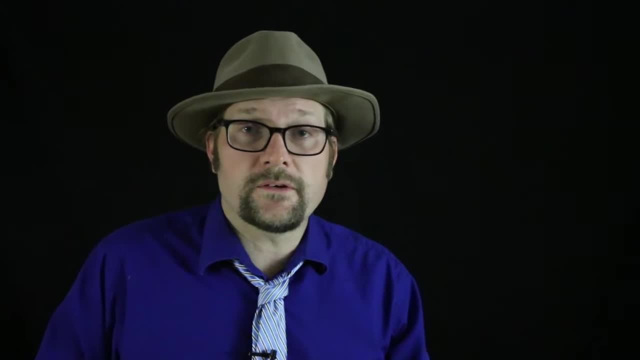 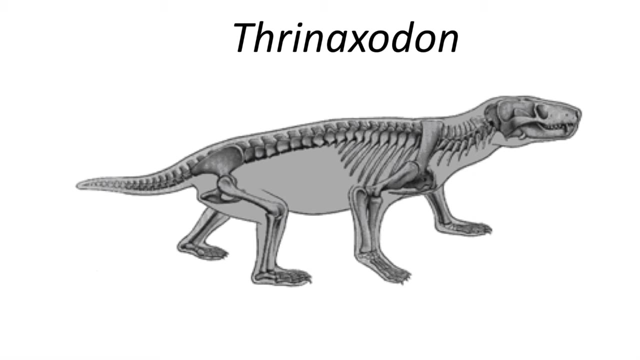 the end-Permian mass extinction. Along with the dinosaurs, The group became successful in the Triassic period. One of the early survivors of the Permian-Triassic extinction was Thyroxodon, which arose from the late-Permian Procynosuchidae family. 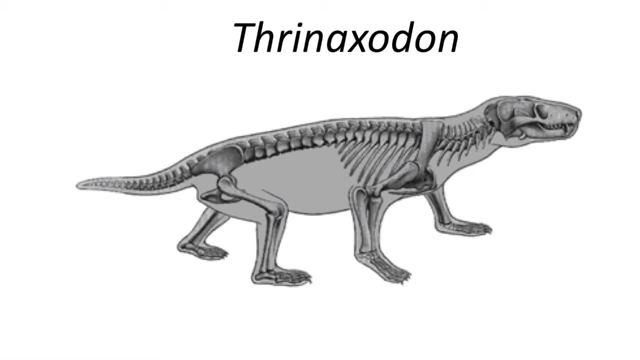 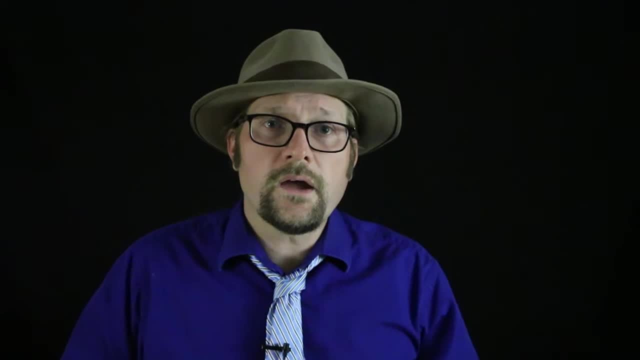 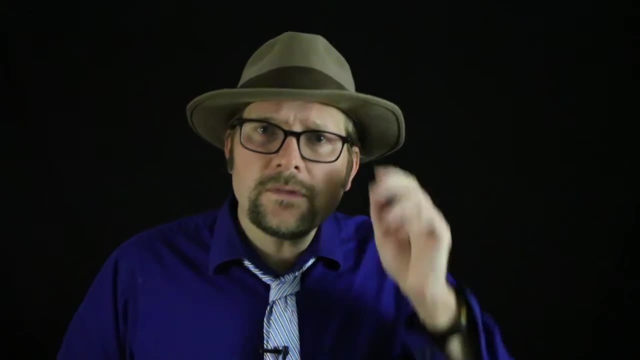 Thyroxodon is well known from some fantastic fossil skeletons from the Karun Basin of South Africa and is worth taking a closer look at. Thyroxodon had a number of characteristics that imply its close relationship with the mammals. It was about the size of a small house cat and exhibited a rather sprawling gait. 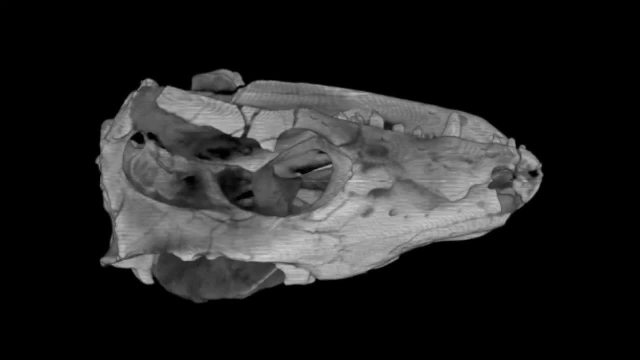 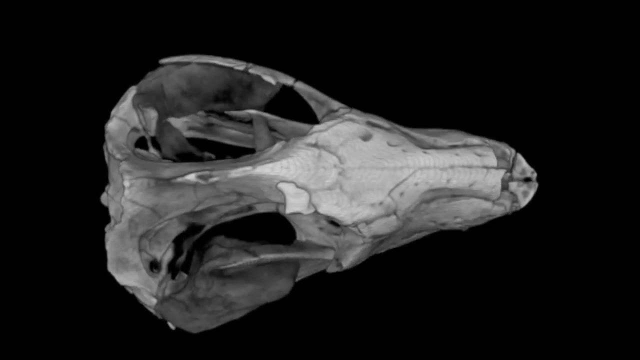 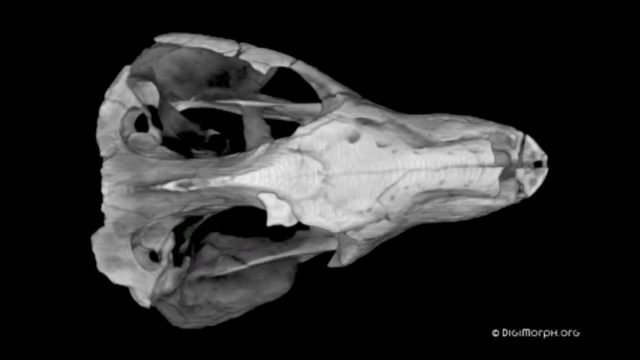 The skull features a large sagittal crest with differentiated teeth into canines and post-canine teeth. The lower jaw features a carotid process, an attachment site for the larger temporalis or adductor muscles of the jaw. The opening of the skull is expanded out into a zygomatic arch or cheekbone. 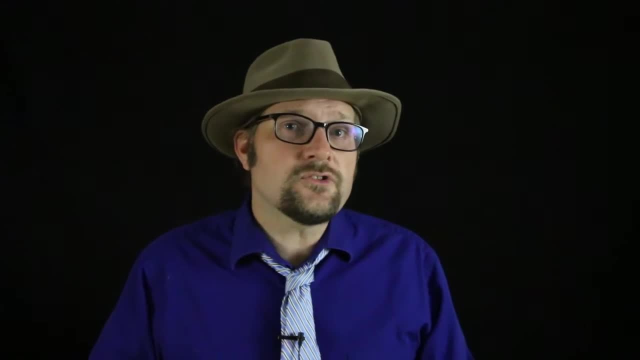 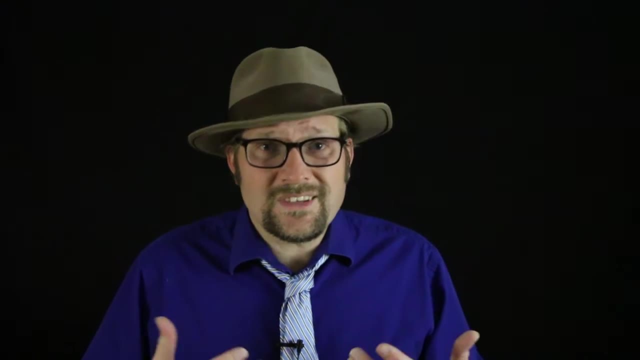 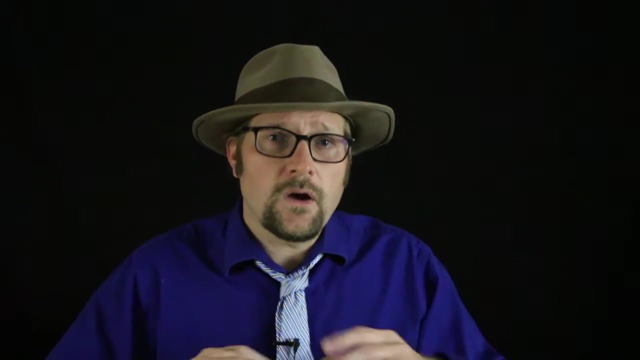 The brain remains small, but the articulation between the neck vertebrae and the skull is achieved with a double occipital condyle, which is a singular condyle in all other reptiles. This double occipital condyle is a unique trait found in all later mammals and helps 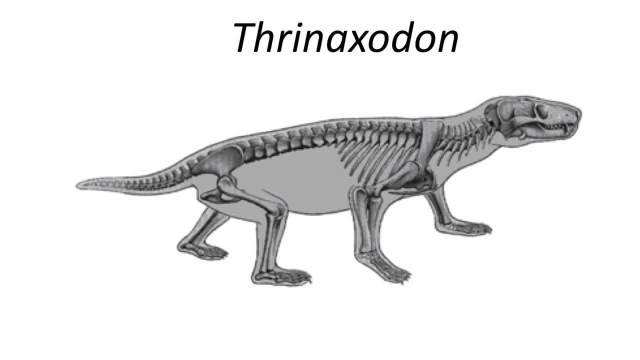 to make a more stable neck joint. Thyroxodon is rather unusual in having robust ribs and a thick vertebral column. It is thought that the robust axial skeleton may have aided in respiration during a period of time when there was very low levels of oxygen in the atmosphere in the early Triassic. 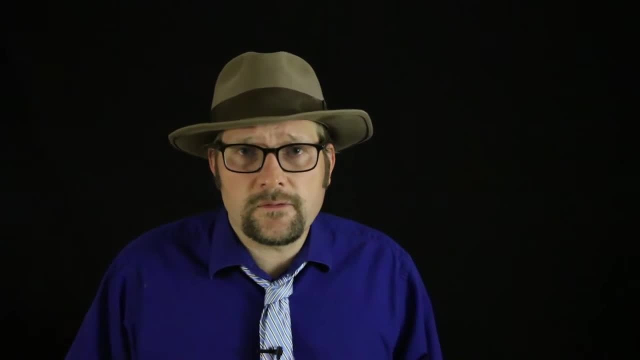 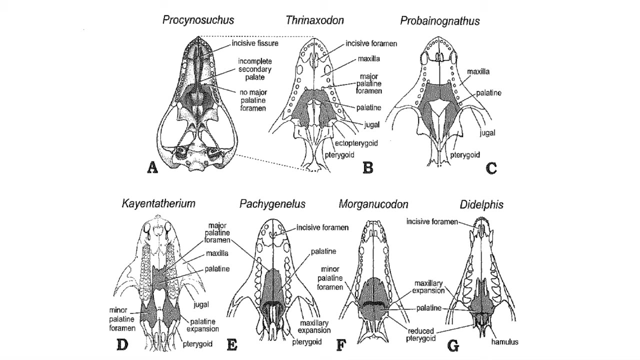 and it helped it to survive the mass extinction at the end of the Permian. Another advanced mammal-like feature can be seen in the roof of the mouth, with the expansion of the palatine bone which forms a longer nasal passage for respiration. 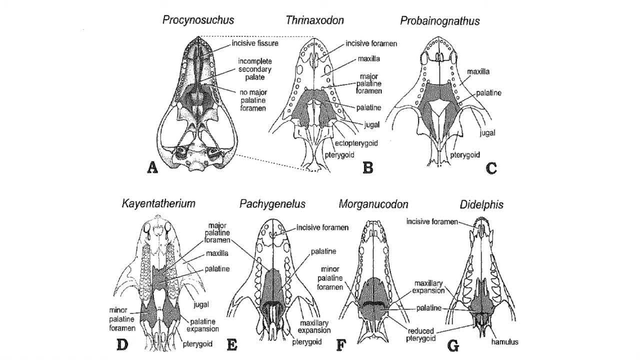 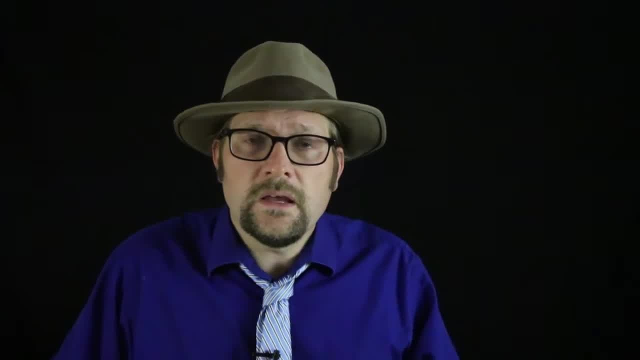 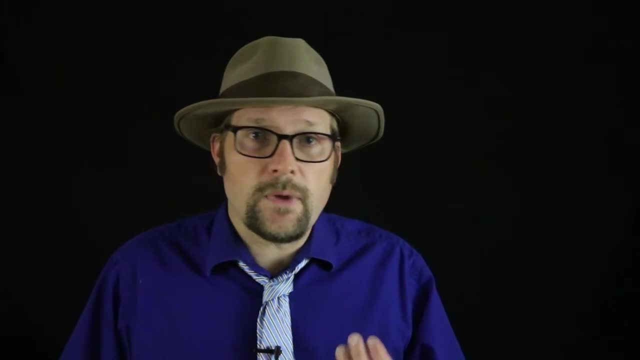 It forms a shelf of bone separating the two openings. This is a secondary palate and would have raised the possibility of suckling in thyroxodon. In later mammals we will see the further expansion of the palatine bone to push the opening between the nasal cavity and the mouth cavity further into the back of the throat. 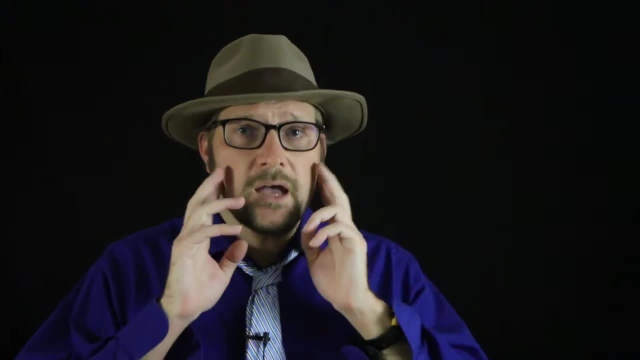 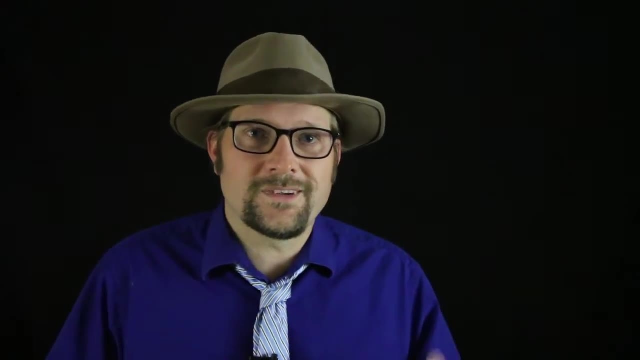 Thyroxodon also features many small foraminifera along the maxilla which have been interpreted as representing nerve and bone. Thyroxodon has been used to justify the reconstruction of thyroxodon as a furry proto-mammal, although direct fossil evidence for fur is not found until the Jurassic. Cynodons were successful during the Triassic and into the early Jurassic, with several groups splitting off. Some became herbivores, such as the gonfiadontidae, which includes two groups, the diadiadontidae. 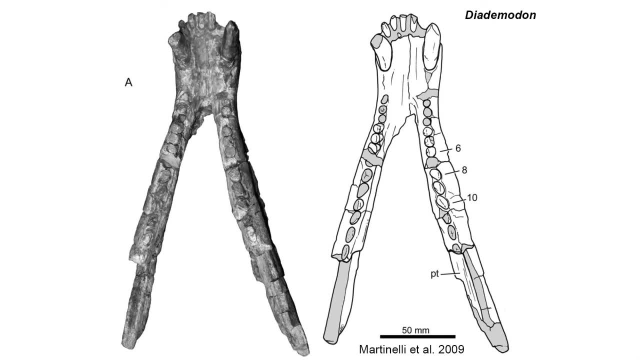 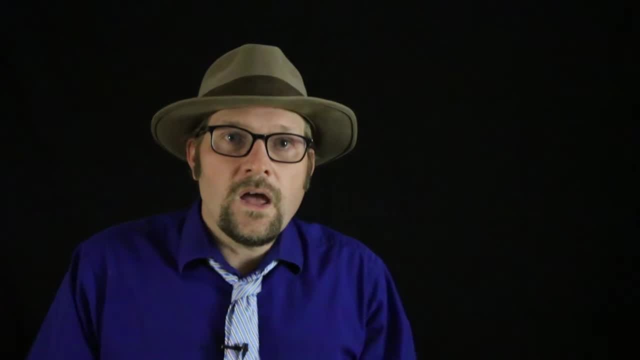 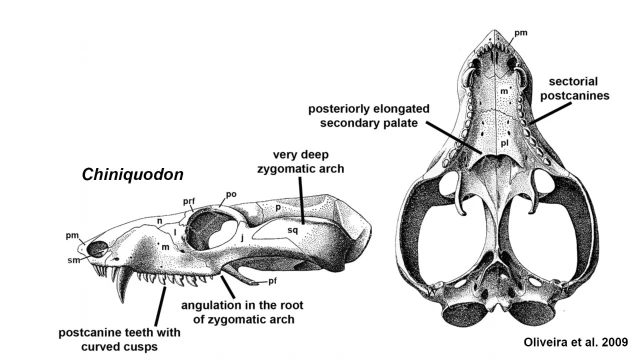 and the diadiadontidae. Another group of triassic cynodons are the chinequiadontidae, which are often grouped with the probanthognathidae, a group more closely related to modern mammals. These animals were carnivorous and feature a much more expanded secondary palate. 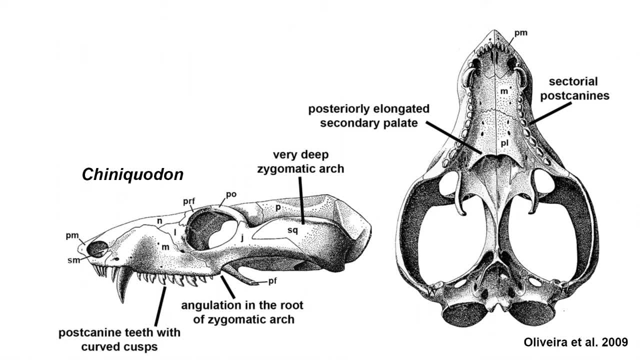 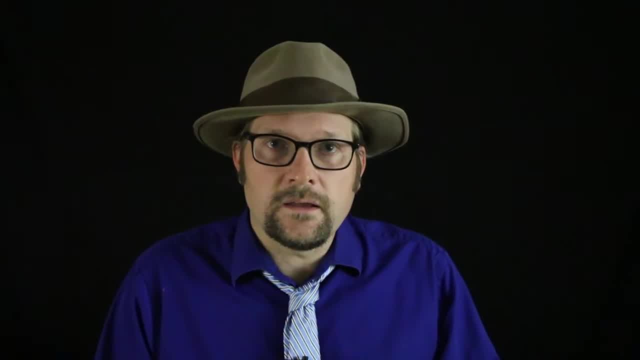 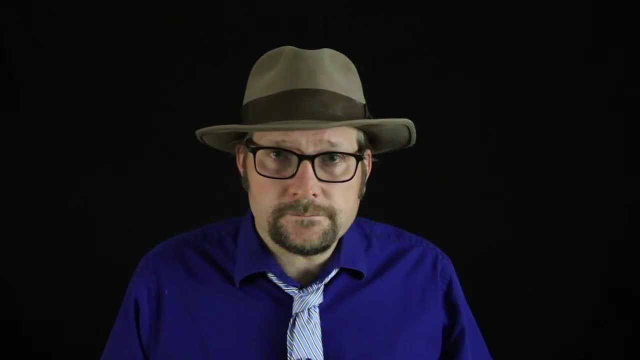 They have teeth with curved cusps, a very deep zygomatic arch and a tiny brain case. The probanthognathidae are another group of small carnivorous proto-mammals that lived during the Triassic. They had by far the most well-developed secondary palate and were even more mammal-like. 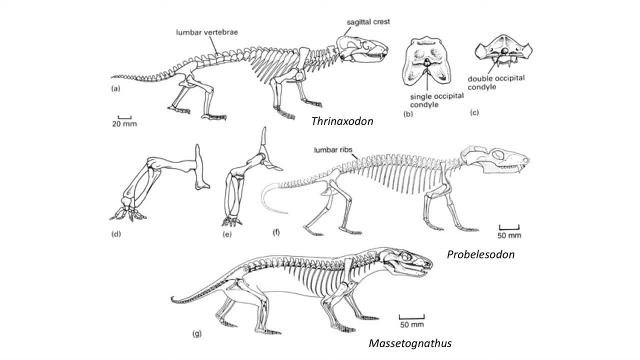 The ribs were reduced to those in the thoracic region, and within this group there might have been the first signs of a diaphragm, a sheet of muscle tissue that helps expand the lung cavity during breathing, and would have helped mammals that achieved a higher. 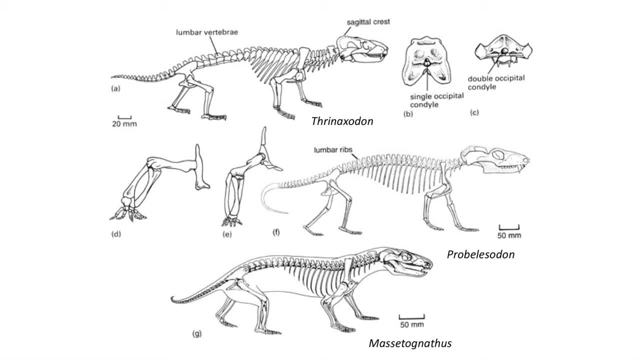 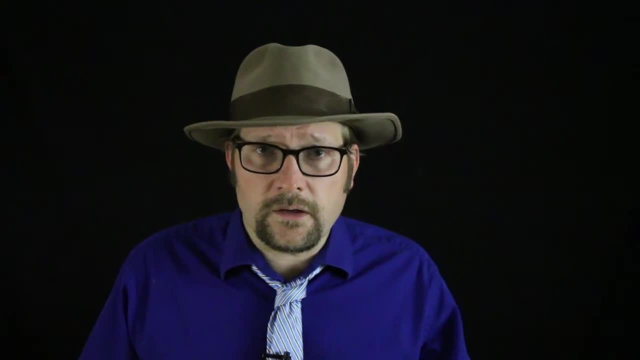 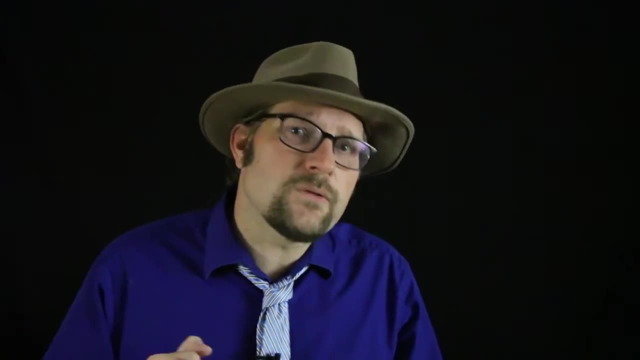 melabolic rate and endothermic thermoregulation. These more advanced forms featured a more erect skeleton than those found in Thoraxodon. Two more advanced groups of cynodonts appear near the end of the Triassic and extend into the early Jurassic: the Trichelodontidae and the Trichelodontidae. 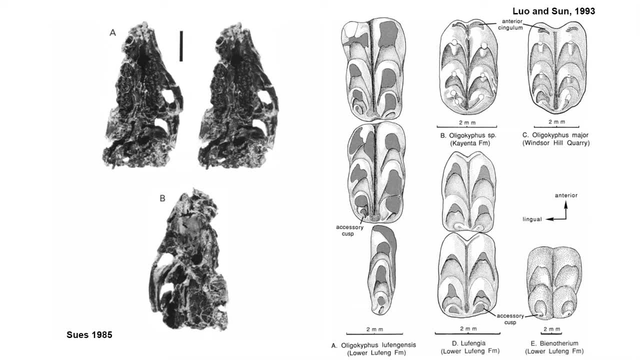 The Trichelodontidae are known from South America and Africa and they feature three cusps on the post-canine teeth and feature wide zygomatic arches and a robust lower jaw. The Trichelodontidae are a better known group, with a number of skeletons from around the. 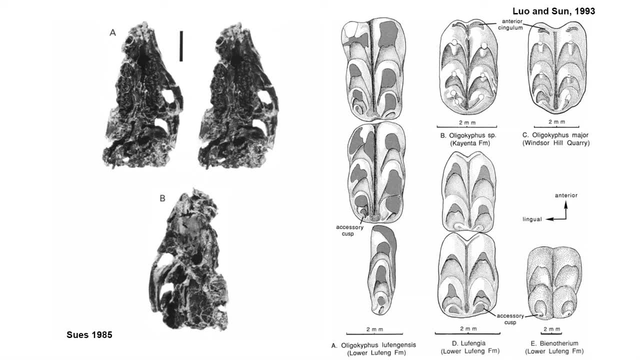 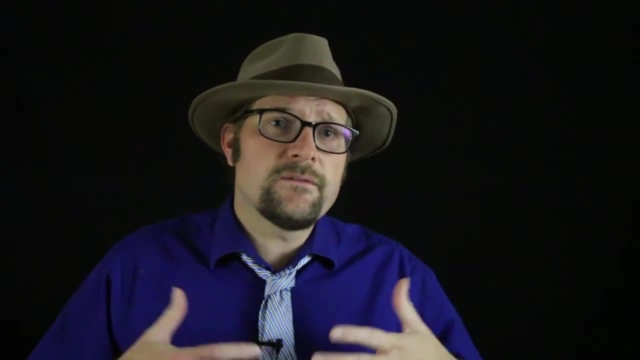 world. The Trichelodontidae feature really bizarre teeth. They have three lobes that interlock between the upper and lower teeth to produce a grinding surface for chewing. The skulls are rather large in proportion to the skeleton. They have very narrow brain cases and large zygomatic arches for large chewing muscles.